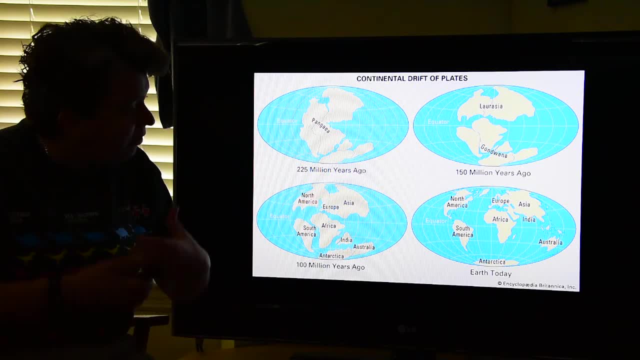 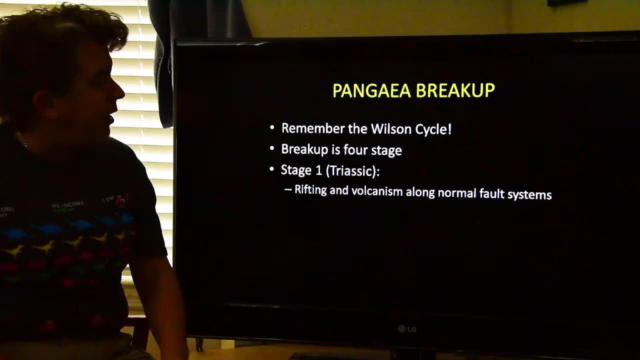 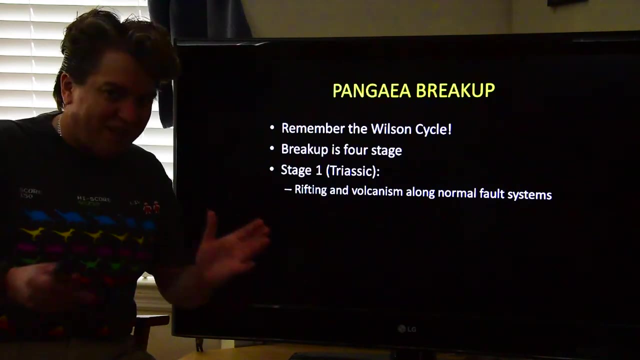 When we were looking at the Paleozoic, we were looking at how Pangea came together. Now it's going to break apart to give us the Earth we know of today. And so just remember the whole Wilson Cycle thing of ocean bases open and then they close and then they open again. 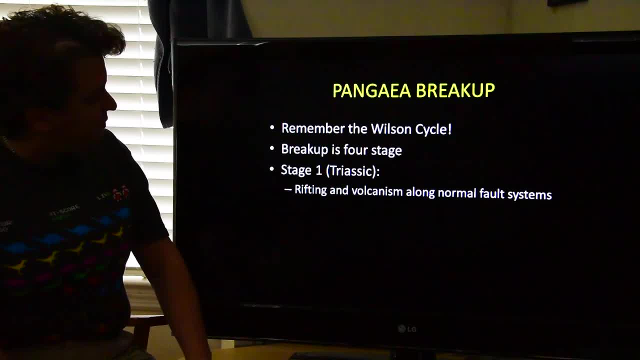 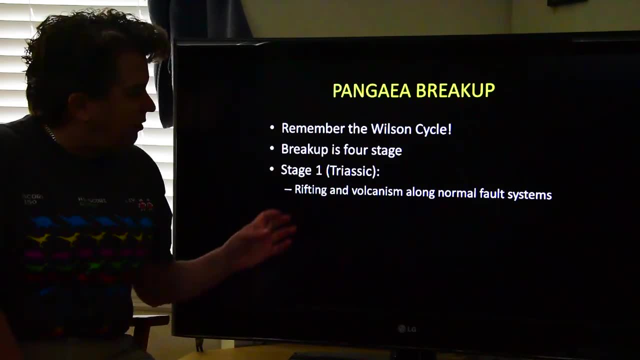 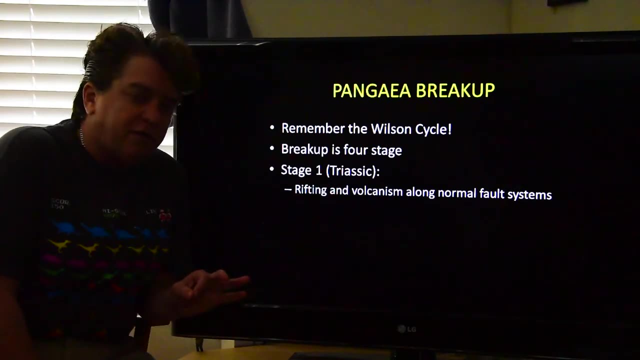 Well, we're at the opening of an ocean basin now And the breakup of Pangea follows about four unique stages And in the Triassic. in stage one, we have rifting and volcanism along normal fault systems- Remember divergent plate boundary- we get a continental rift developing. 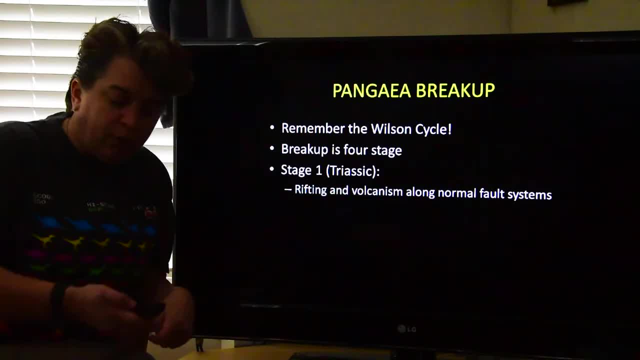 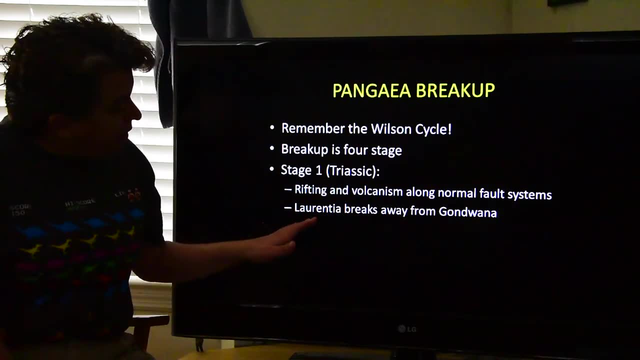 Normal faults are typical where you have tensional pull-apart stresses. So we start seeing these rift systems develop in Pangea. Laurentia breaks away from Gondwana, So North America is breaking away, So we're at the opening of the Mesozoic. 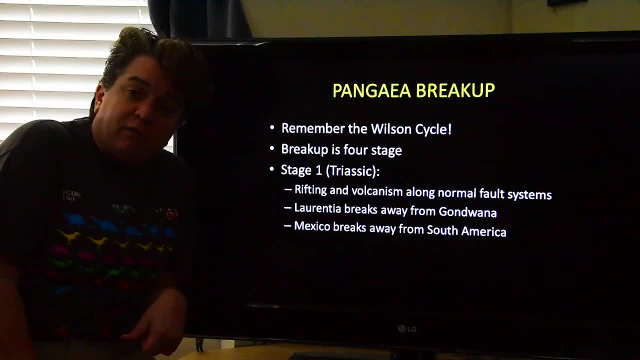 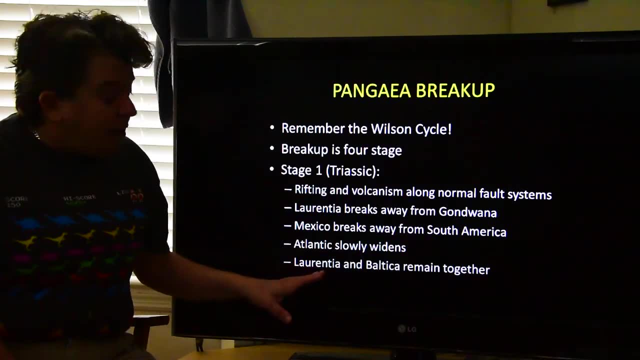 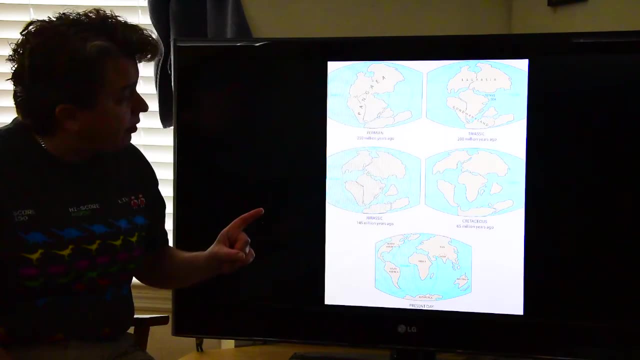 And the Atlantic breaks away from the southern continents, Mexico breaks away from South America, And the Atlantic slowly starts widening At this time though Laurentia and Baltica, so you can think North America and Europe are still stuck together. So this was when Pangea was all together in the late Paleozoic. 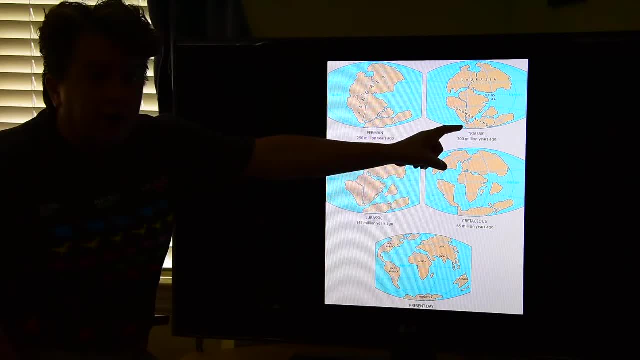 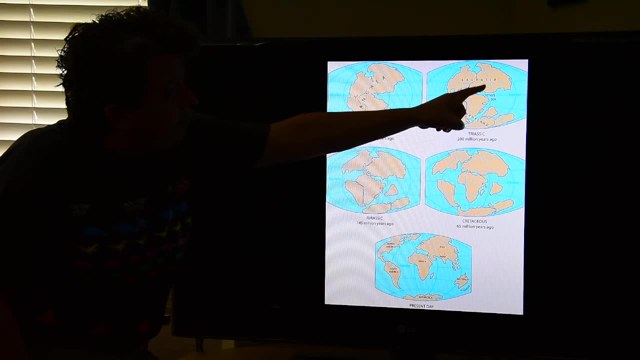 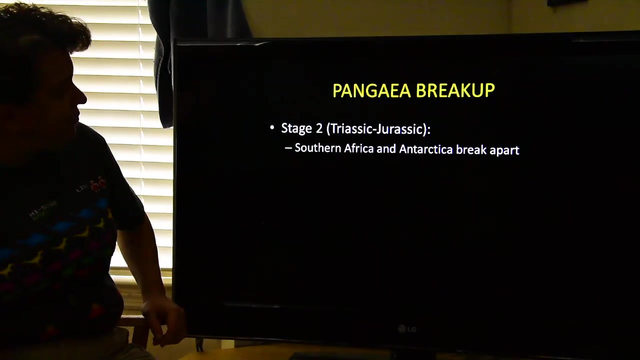 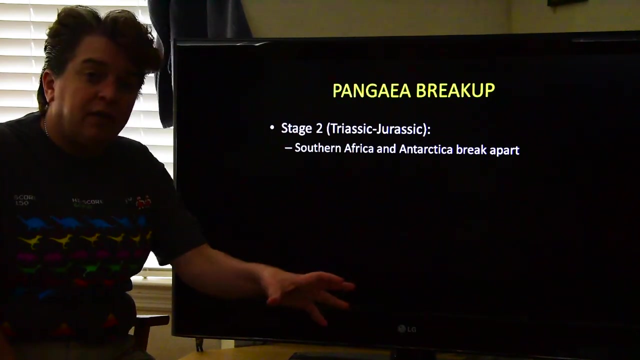 In this beginning of rifting we see that Laurentia and Europe are still stuck together, but Laurentia is breaking away from these southern continents. So we're starting to get the Atlantic Ocean forming right there, just starting to widen. Now in stage two, in the next part of breakup, that is, in the late Triassic into the Jurassic, 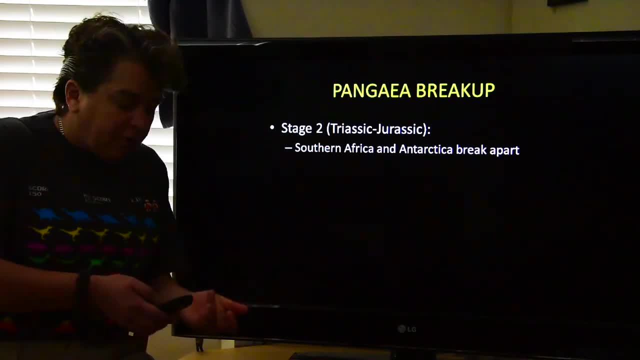 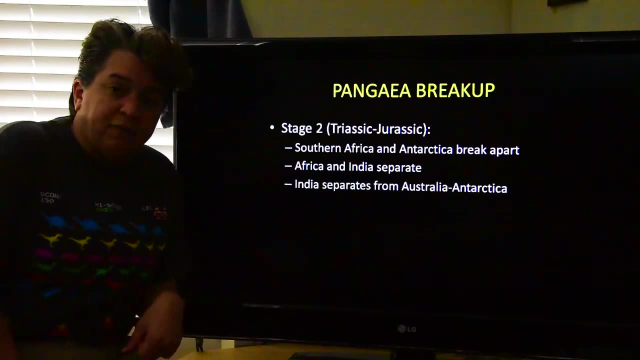 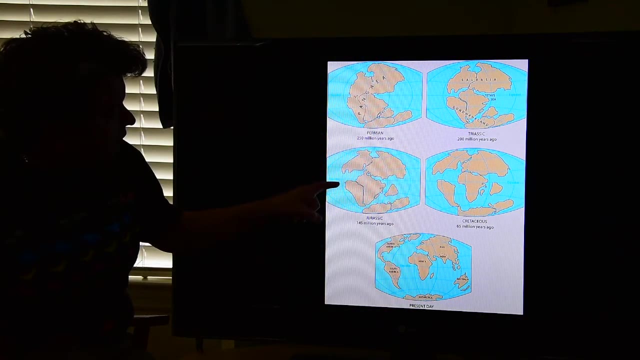 Southern Africa is breaking away from the Atlantic, South America and Antarctica break apart. Africa separates from India, India separates from Australia and Antarctica. Those two continents are still stuck together, And so that's what we're kind of seeing right here. The Atlantic is widening. 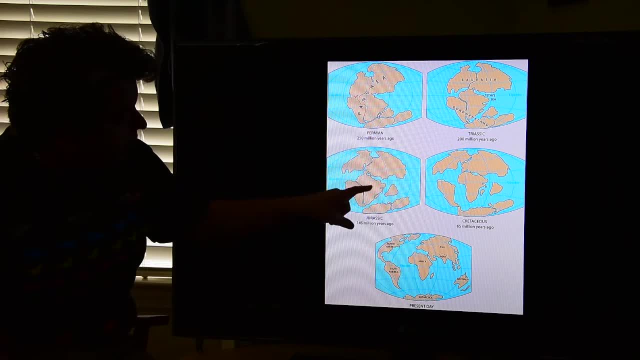 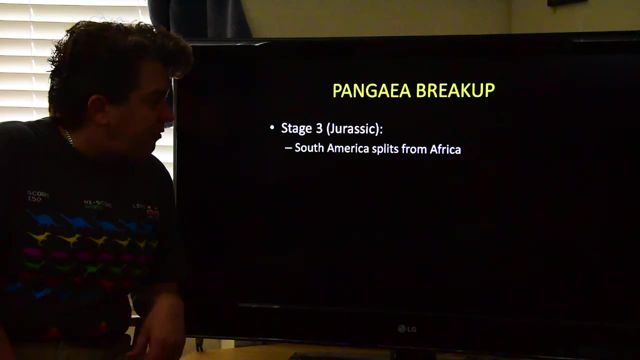 Europe and North America are still together. South America and Africa are stuck together, But India is starting to split apart And these have been split apart. These two continents have split from Antarctica And then, in stage three in the Jurassic, South America starts splitting away from Africa. 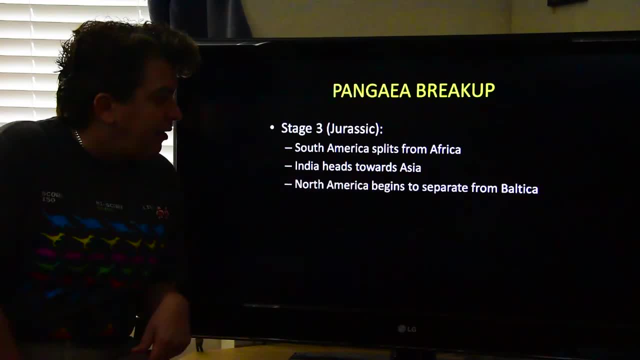 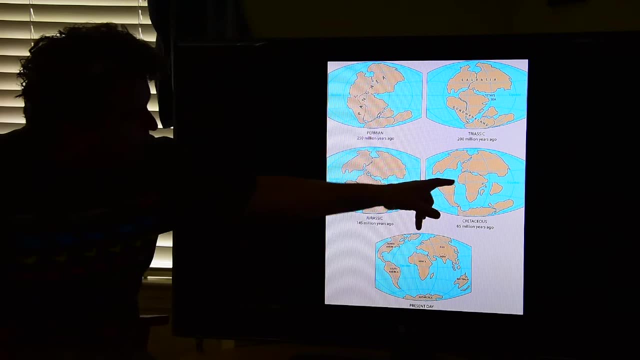 India is starting to head up towards Asia. North America begins to separate from Baltica And so we're kind of in between these two where these are splitting. We're starting to get North America and Baltica splitting apart. India booking traveling really fast up towards Asia. 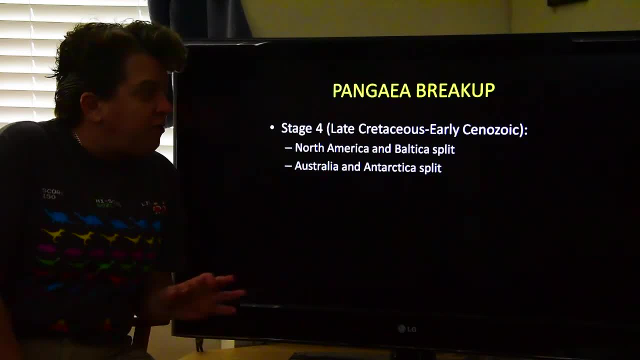 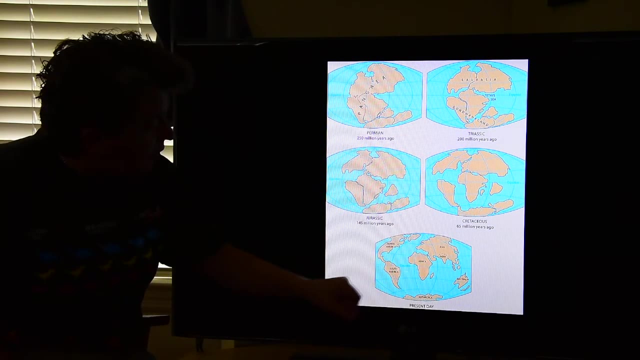 And then in stage four, the late Cretaceous to the very early Cenozoic, North America and Baltica finally split apart. Australia and Antarctica finally split. So these guys are going to split off And Australia is going to move into its current position. 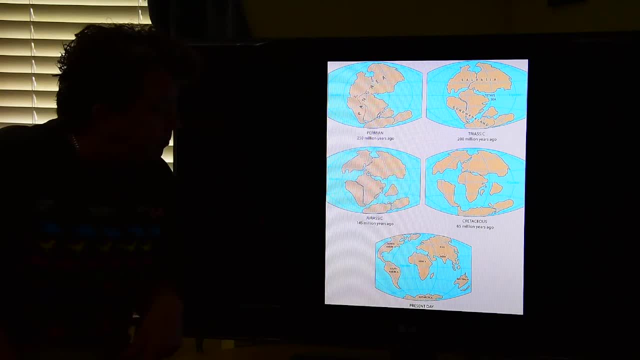 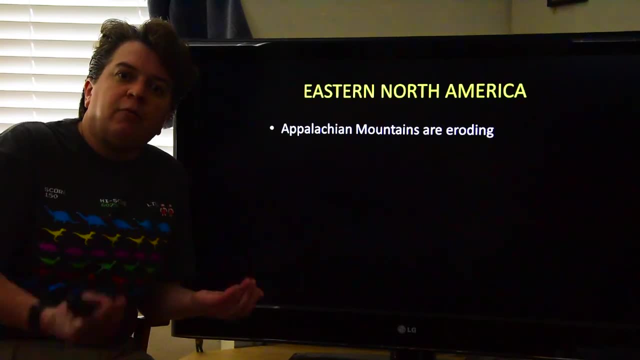 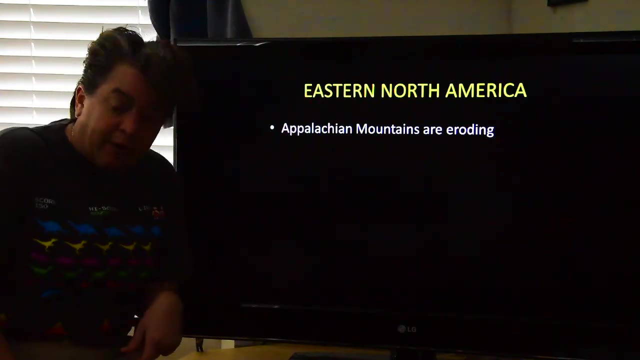 India is going to hit Asia, And so that's our breakup of pandemics. It takes quite a number of millions of years for these different continents basically to tear away from each other and move to their modern positions Now let's focus especially, then, on North America. 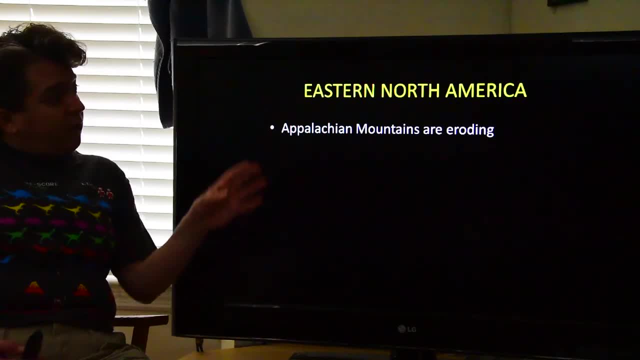 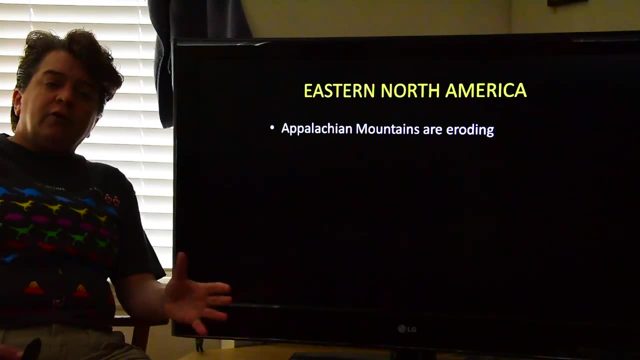 what's happening on our continent? Well, in Eastern North America we have those Appalachian Mountains are eroding right. They formed during the time when Pangea happened. Now Pangea was assembling And now Pangea is breaking apart. 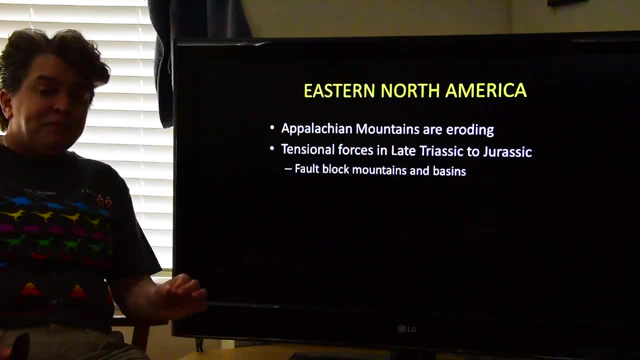 And these things are simply slowly eroding away. But remember: North America is eventually going to rift, It's going to split away from Europe, And so we're starting to get some tensional forces in the late Triassic into the Jurassic right. 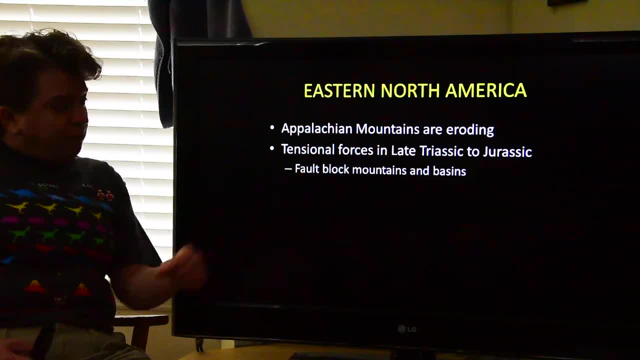 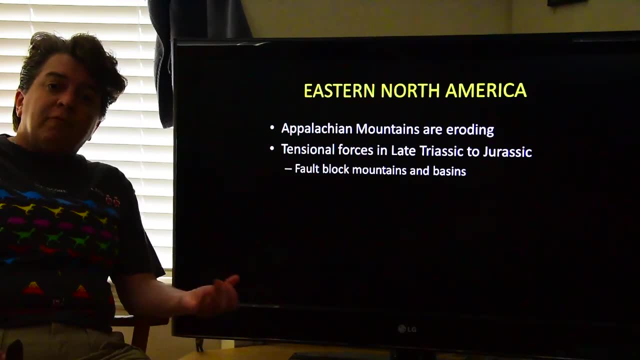 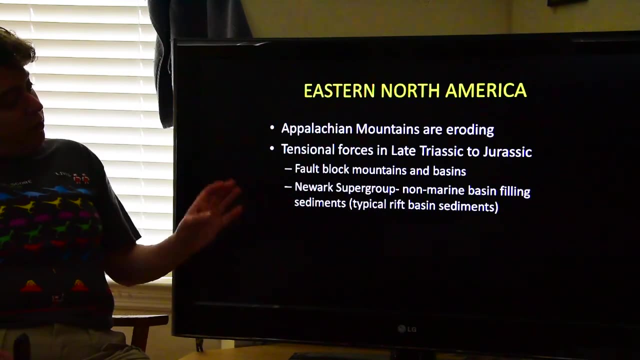 Pull apart forces in the East And some fault block mountains and basins start forming. Remember your Horsts and Grobbins from physical geology. That's what we start seeing on the East Coast of North America, And one of the big rock formations that forms at this time is called the Newark Supergroup. 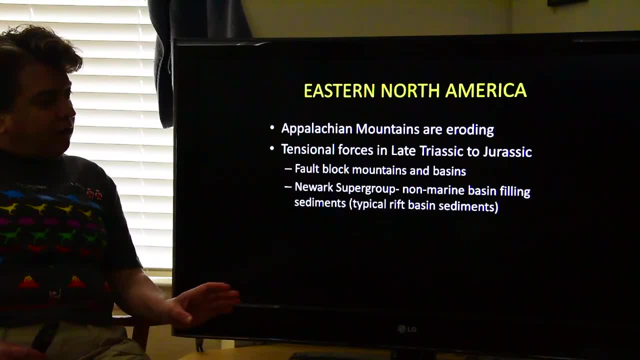 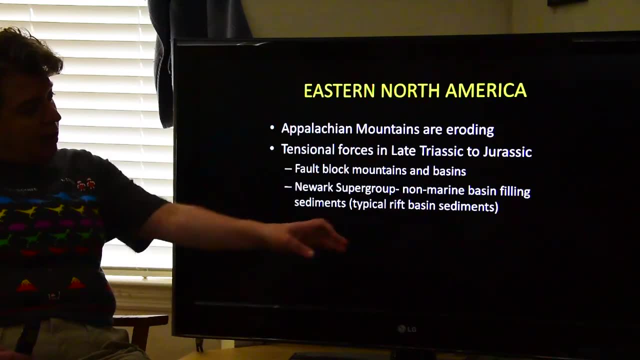 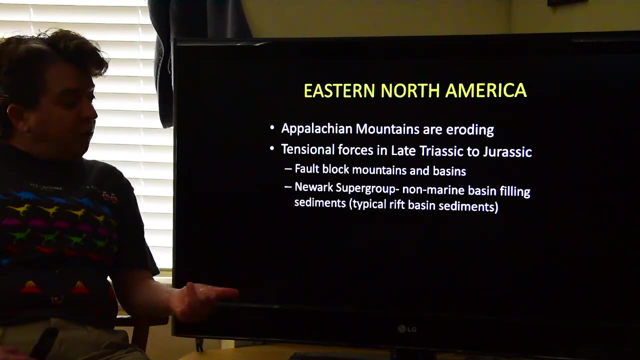 And this includes all sorts of different sediments that were accumulating in these basins, that were developing, And these are non-marines, So these are terrestrial sediments accumulating in those basins And what's interesting is in some of these we have like track waves of dinosaurs and things preserved. 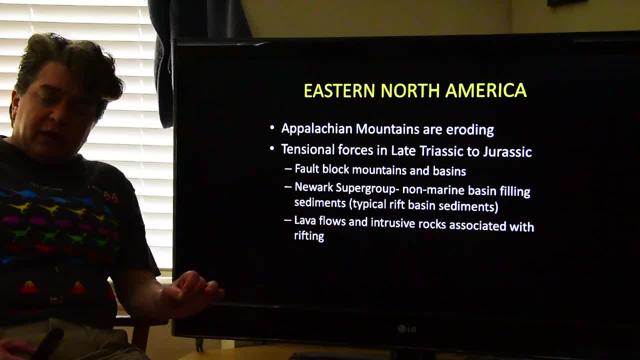 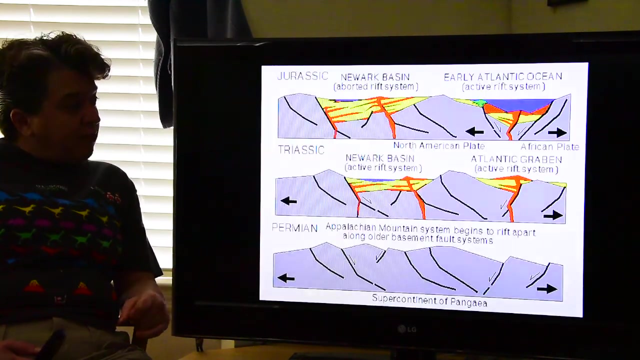 Now, in addition to the sediments accumulating in these basins, we also have volcanic activity, Because when you have rifts developing, you have volcanism And there's, in fact, a number of lava flows And also intrusive igneous rocks found in the Eastern United States that formed during the time of this rifting. 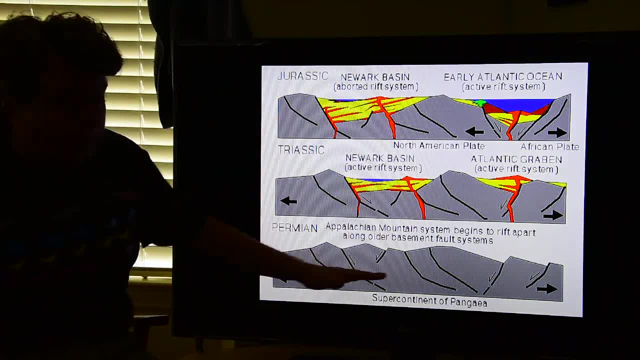 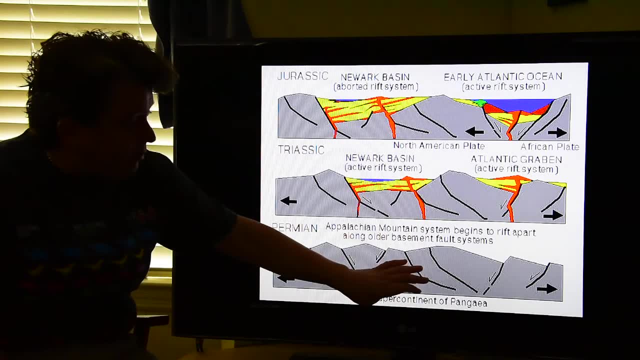 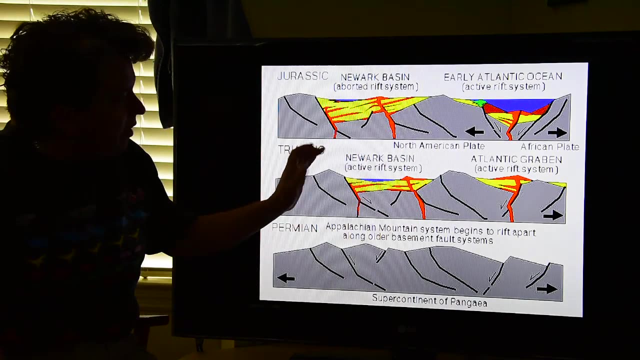 So what we're seeing oldest here is on the bottom. This is the Permian right, Pangaea assembled And we get the Appalachian Mountains forming. But as Pangaea starts breaking apart and we start having the pull apart forces, we start having those Horsts and Grobbins developed right. 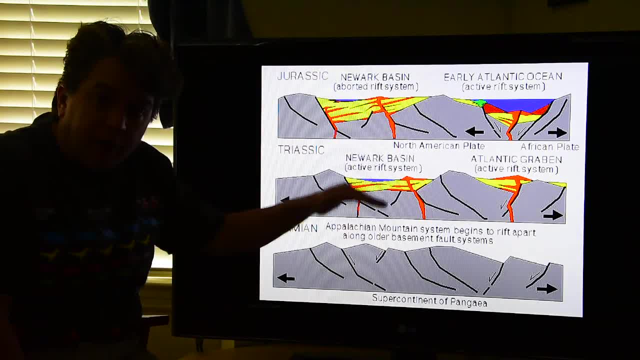 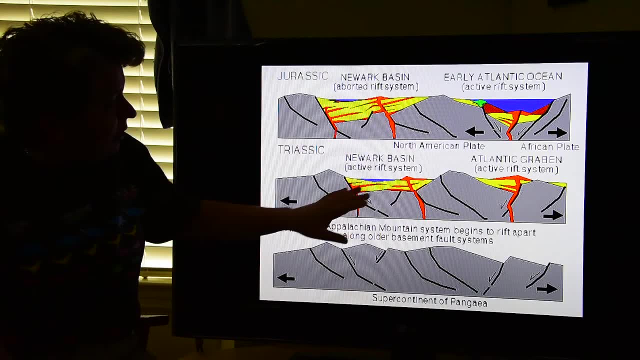 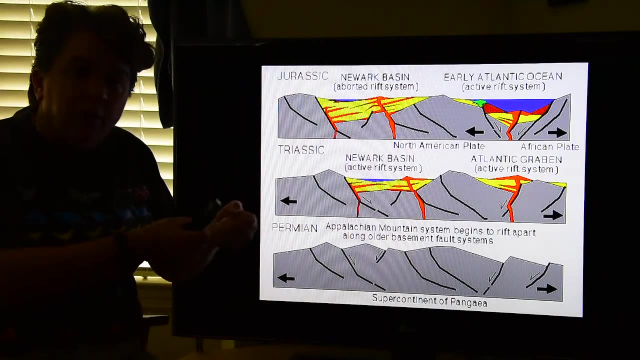 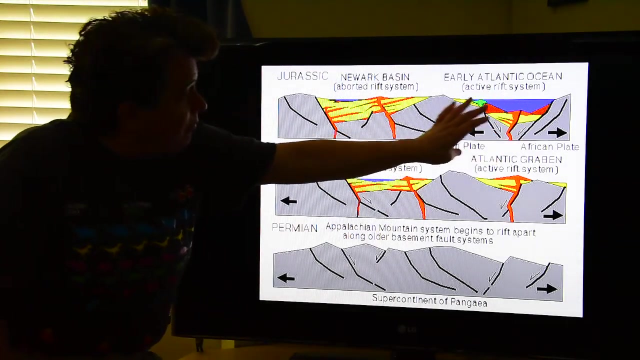 The down-dropped block is called a Grobbin. That's going to form a basin where sediments start accumulating, And that's what we see here. And then, once we get into the Jurassic, this pull apart activity that was happening gets focused where the Atlantic Ocean is rifting apart. 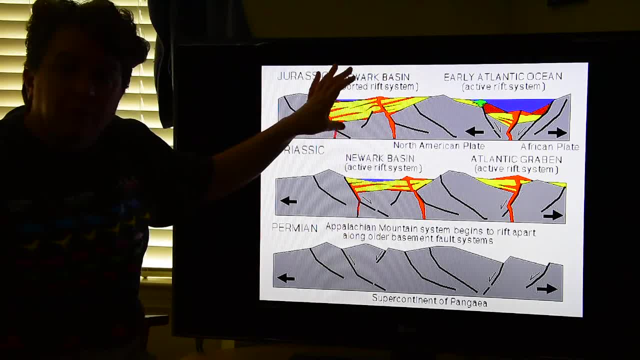 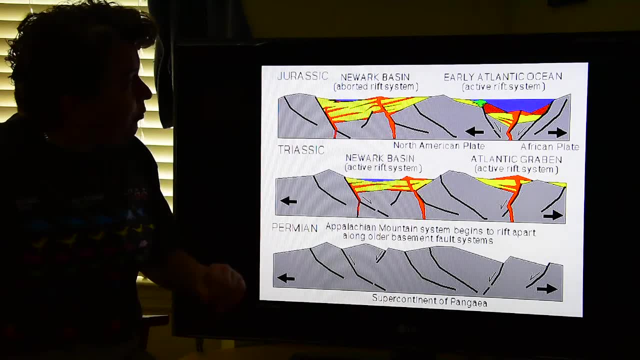 And this is kind of a, they say, an aborted rift system or a failed rift. That's where this Newark supergroup sediments, lots of them, were accumulating And so we have thick sediments, volcanics, in there, And this stopped rifting. 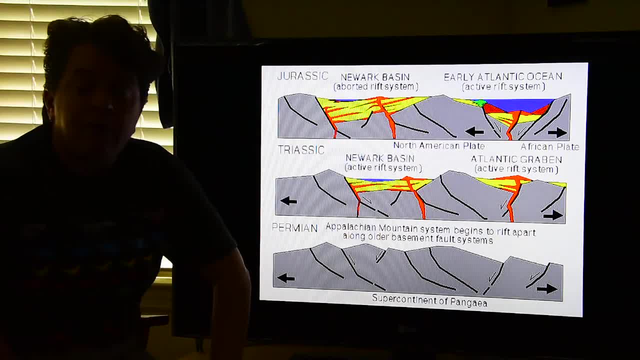 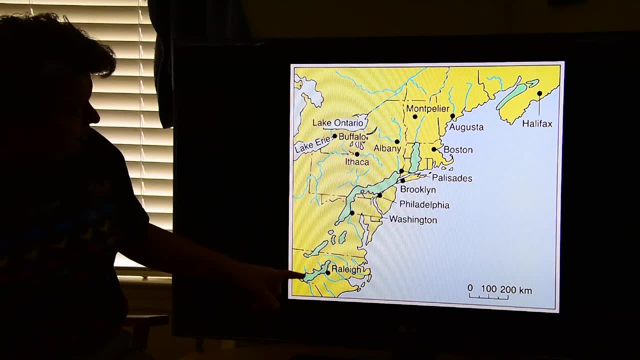 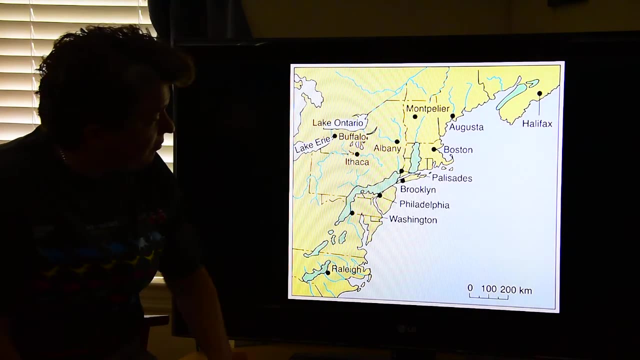 And the rifting really focused in what becomes the Atlantic Ocean. Now, what this diagram is showing, we have the east coast of North America here And in green these are some of the igneous rocks associated with that rifting event. So those are places where you can go to see those igneous rocks. 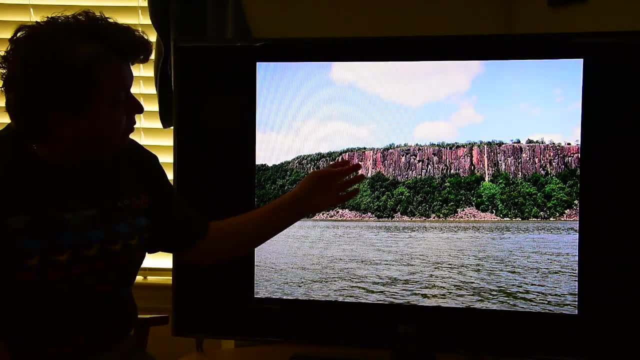 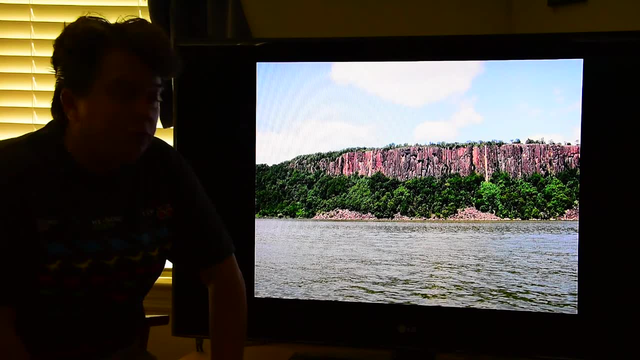 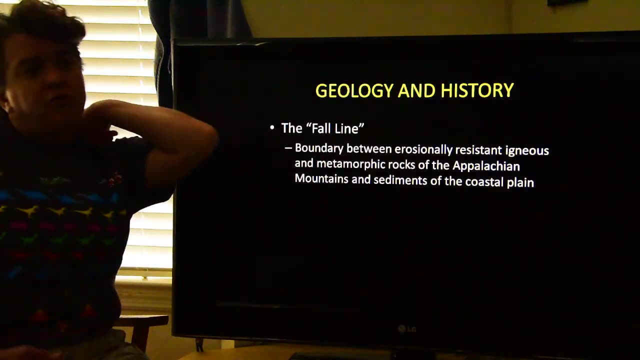 And one of the famous ones is actually along the Hudson River. It's called the Palisades And the Palisades- this was a sill that was intruded into that area associated with that rifting event. Now, geology oftentimes plays a role in human history. 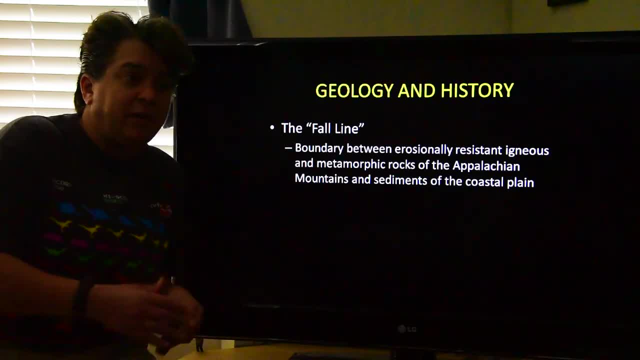 Because geology is basically shaped. Geology is basically shaping the planet we live on, right, And then we have to react to what the planet does or has done in the past. So let's look at one way that geology has shaped American history. 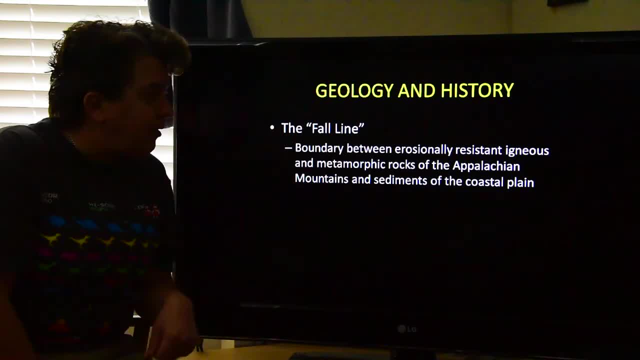 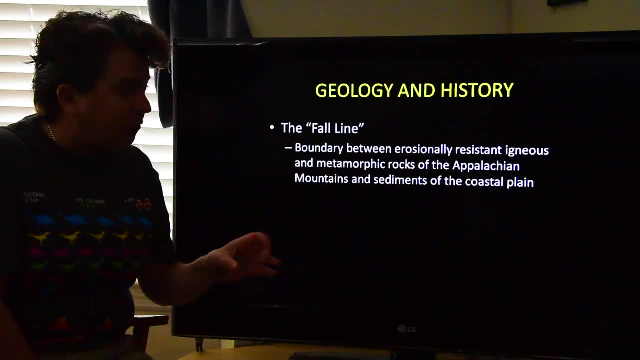 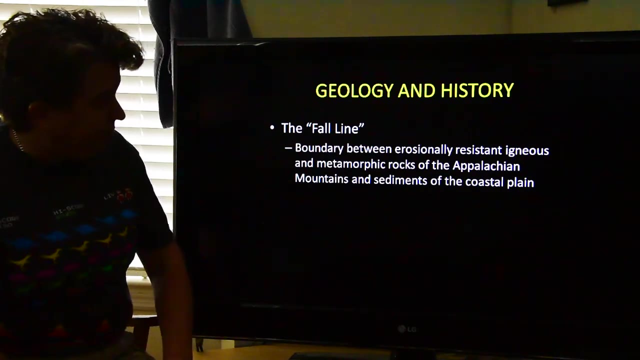 There's something known as the fall line, And the fall line is the boundary between erosionally resistant, igneous and metamorphic rocks of the Appalachian Mountains And then these easier to erode sediments, And the fall line is the boundary between erosionally resistant, igneous and metamorphic rocks of the coastal plain. 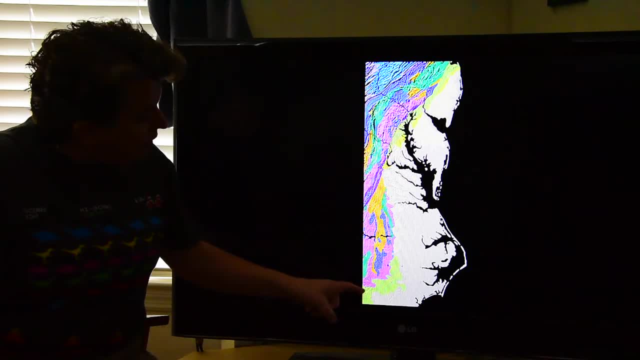 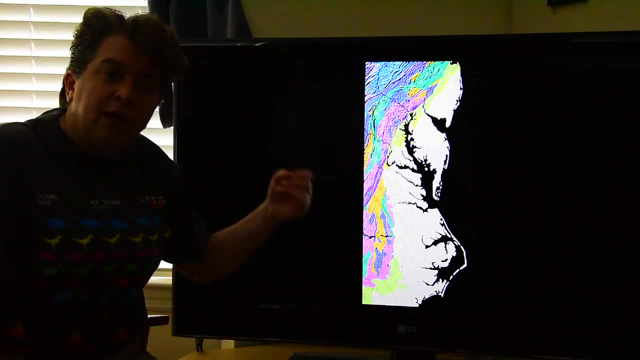 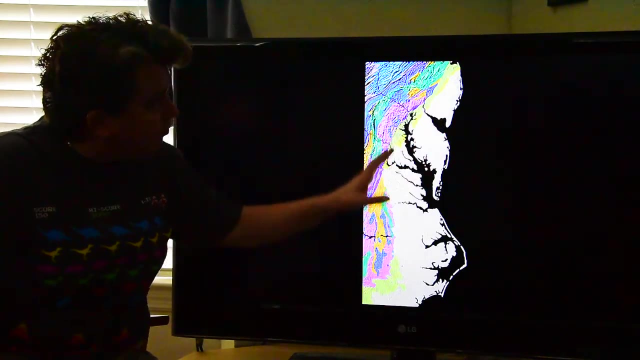 And you can actually see that on this geologic map here, These colorful areas right And the purples and greens and blues, That's all our igneous and metamorphic rocks that are difficult to weather and erode, And then in these yellows and kind of grays, that's the coastal plain area. 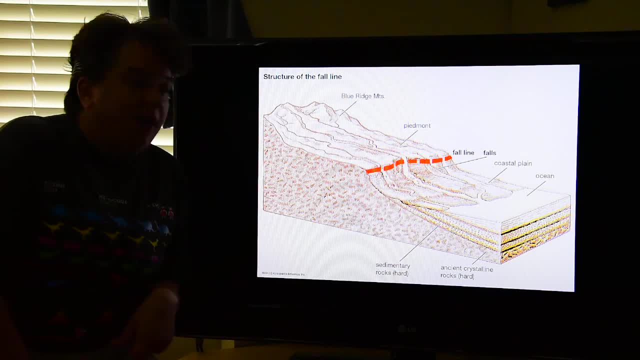 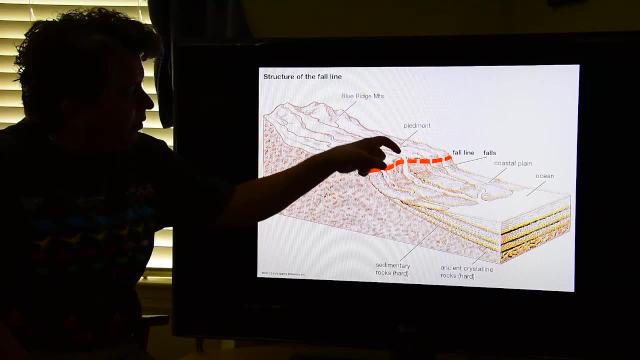 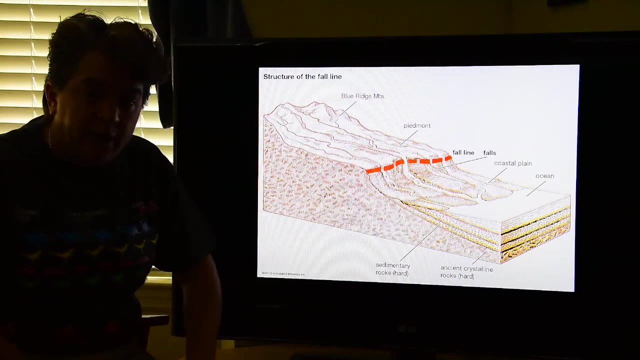 And why this is called the fall line is because we see a sudden elevation. There's a sudden elevation change there right Hard to weather and erode. Then there's the fall line where we have these waterfalls and stuff And then we have our coastal plain area. 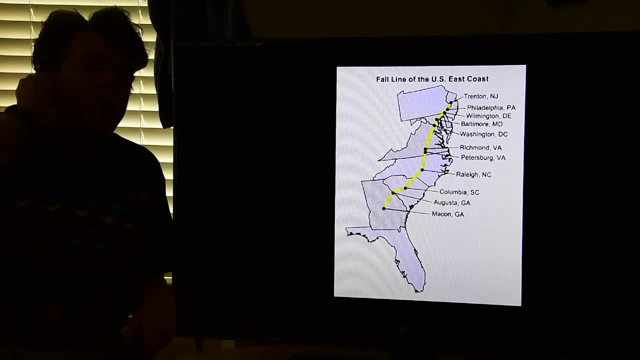 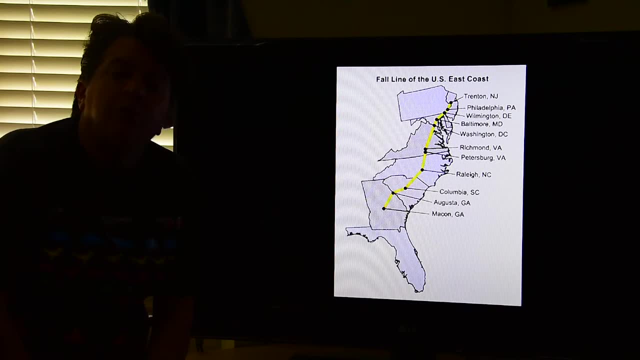 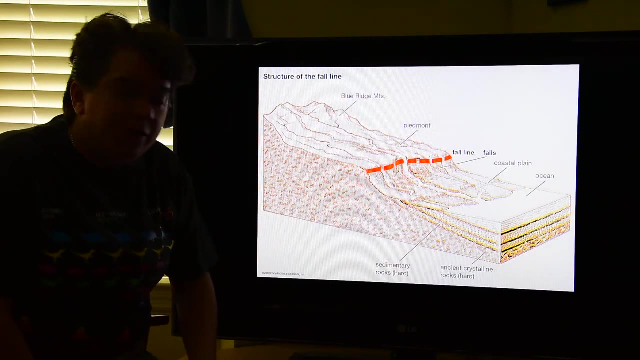 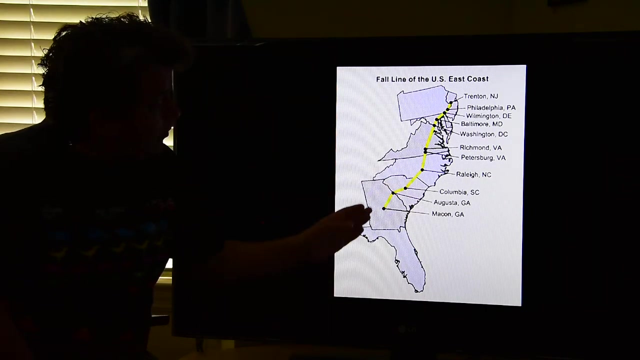 So what did this have to do with history? Well, when North America was settled, one of the main power sources were water wheels- And it's great to power a water wheel where you have this change in elevation. And so many of our colonial cities in the United States were founded on the fall line. 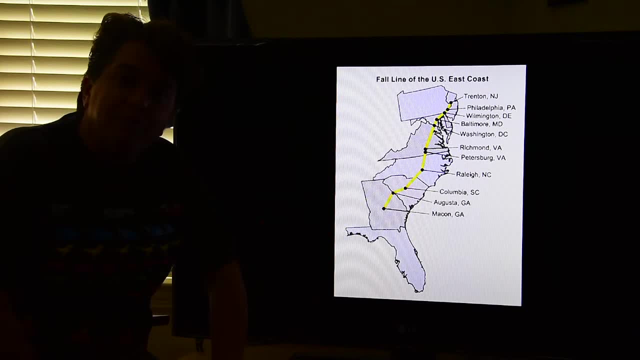 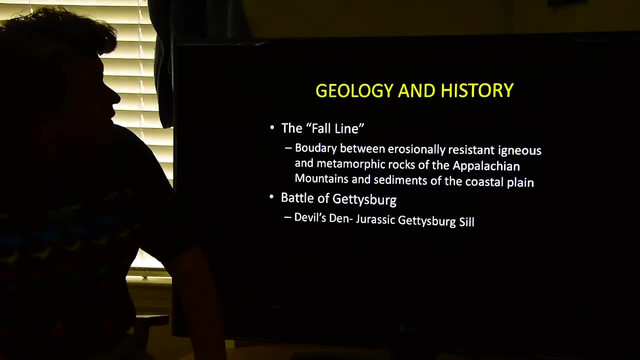 because it was a convenient place, since it had a ready energy supply for those settlers. And so you can see, right here is the fall line and there's a bunch of these famous cities from colonial times in America, Now the British Empire, Now the British Empire. 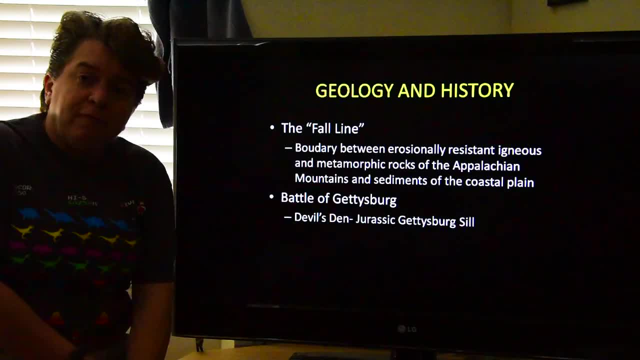 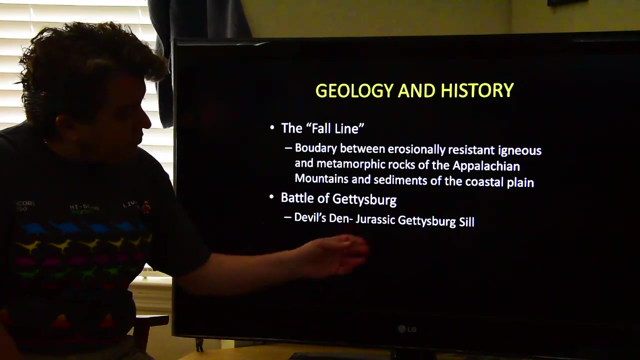 The breakup of Pangea also affected the United States in the American Civil War. in the Battle of Gettysburg, Some of the very hard fought areas in Gettysburg were in a place called Devil's Den, And Devil's Den is the Jurassic Age, Gettysburg sill. So what you have? this is Devil's Den. This is igneous rocks that were in place in that rifting time, And this is where there were a number of Confederate forces, And they set up many of their sharpshooters there to shoot at the Union. 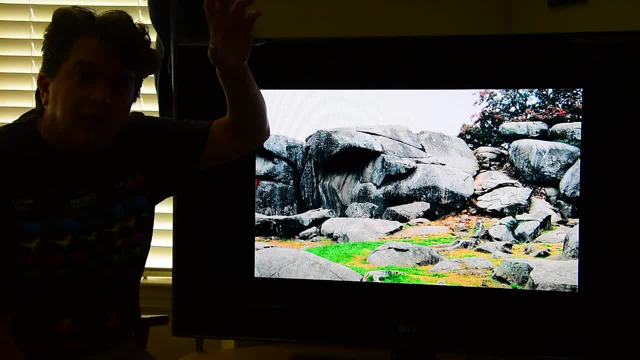 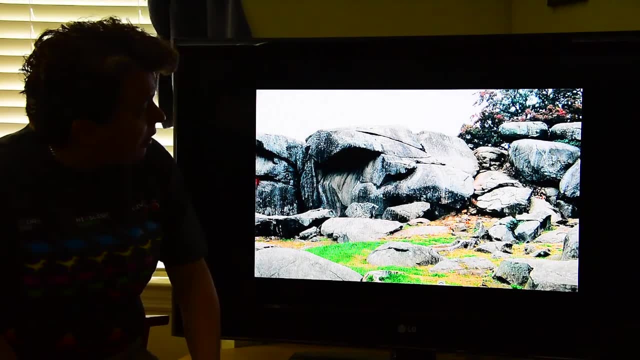 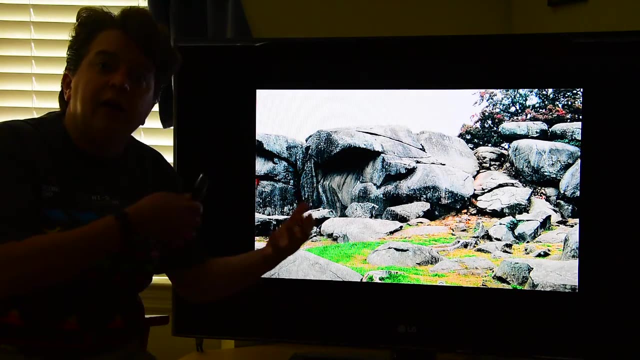 especially the officers, who were stationed on a hill which was a very well defended piece of land for the Union, And so, in any case, that's the Battle of Gettysburg, in part, was shaped by these igneous rocks that were created as Pangea ended up breaking apart. 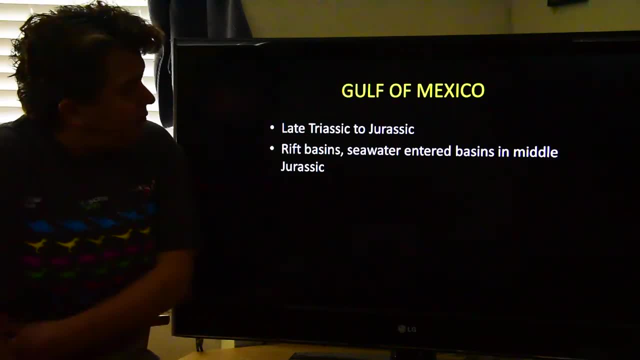 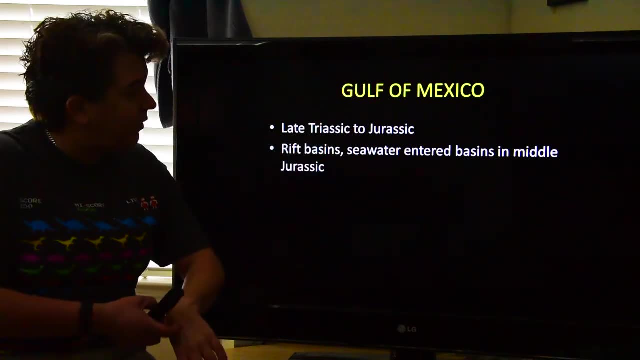 Now, what was happening in our neck of the woods in the Mesozoic? Well, let's look at the Gulf of Mexico, And this is going to be forming in the late Triassic into the Jurassic, as we're splitting continents apart, And so, again, we're going to be in the Gulf of Mexico. 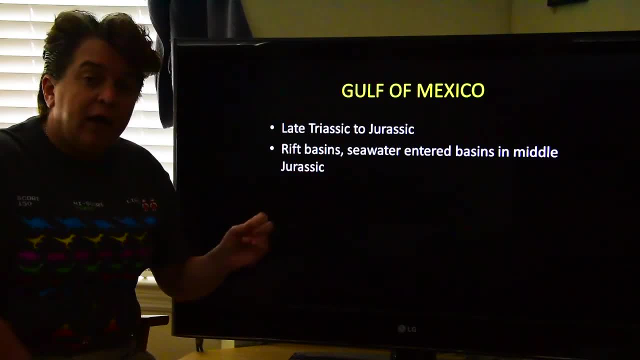 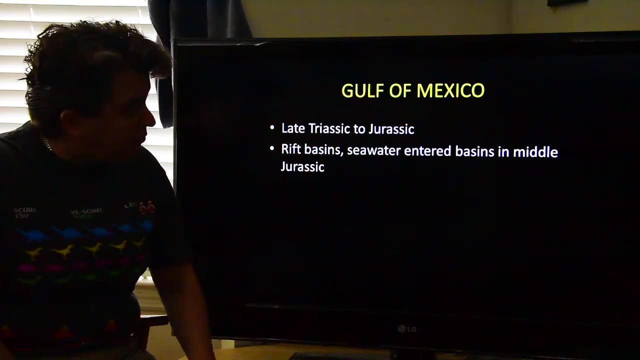 And so again, we're going to be in the Gulf of Mexico, We're going to get rift basins developing here And eventually, as this pull apart continued, sea water entered those basins. So we're having salt water there by the middle Jurassic. 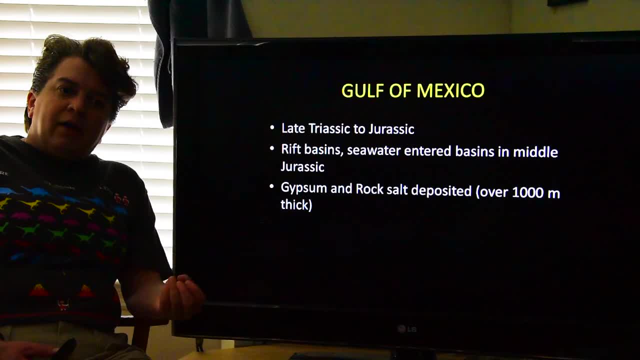